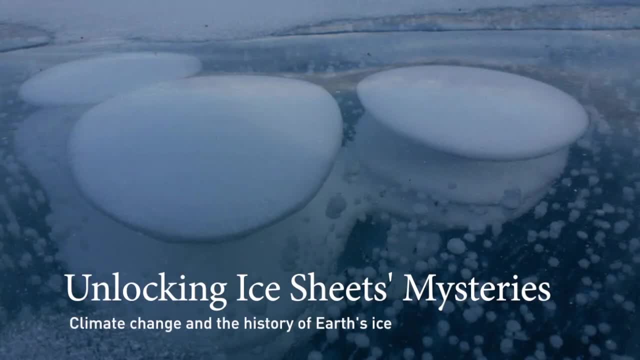 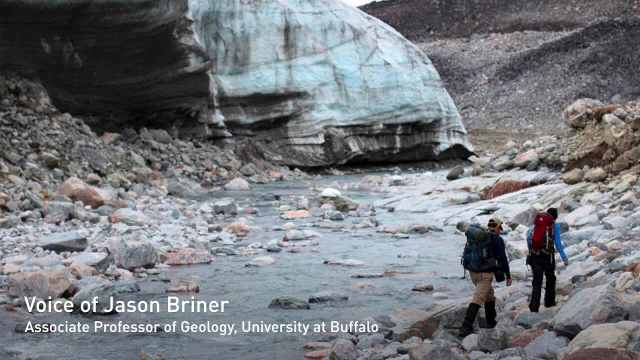 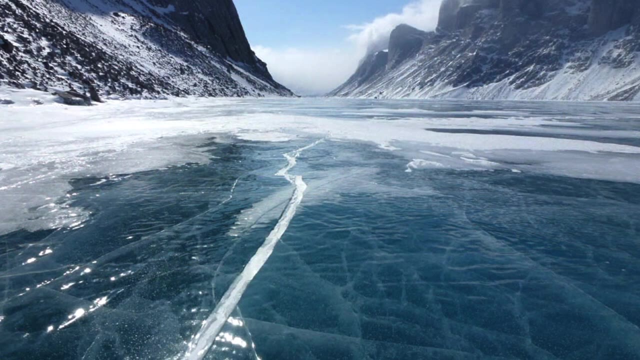 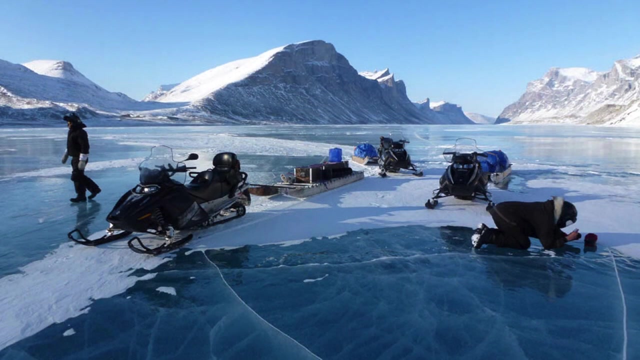 We're learning more and more about how ice sheets are changing. today, The change that's taking place in Greenland and Antarctica is really highly variable, And what's uncertain, given the relatively short duration over which we've been monitoring these changes, is we don't know necessarily what the ice sheet did or how the ice sheet 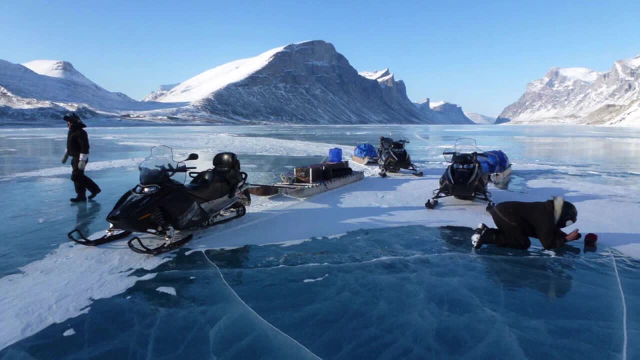 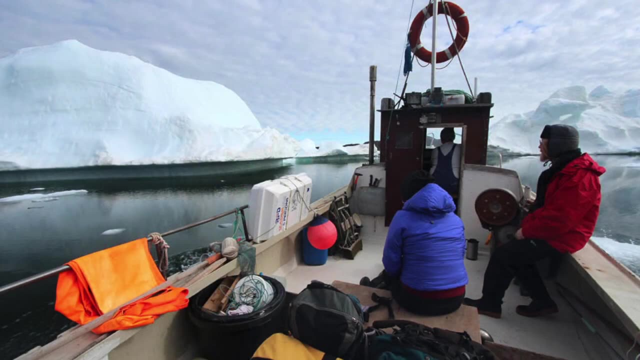 responded to climate change in the geologic past. We don't have direct observations or knowledge of what the ice sheet did prior to a hundred years ago, for example, or a thousand years ago. What my team has been working on is to reconstruct, basically past changes of the Greenland ice. 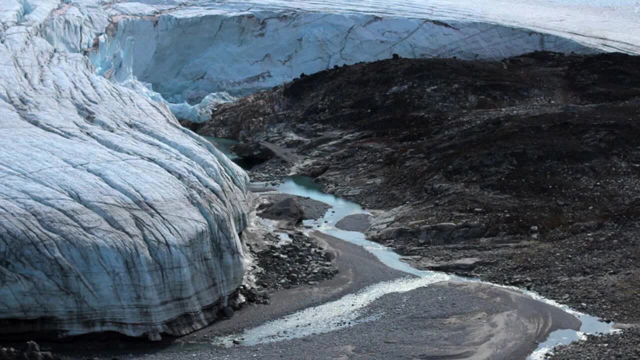 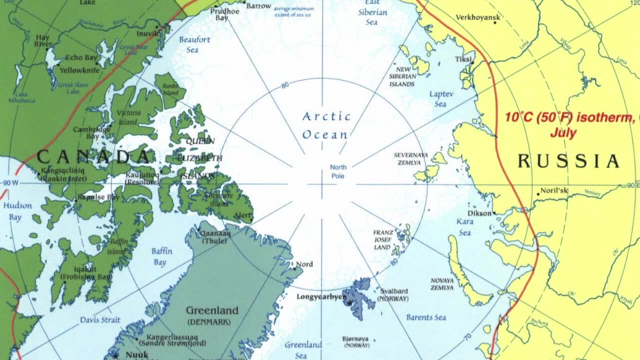 sheet margin. We look at features and deposits that the ice sheet has created, that are still on the landscape today. We can go to Greenland and we can go to Arctic Canada, to Baffin Island, and see these traces of the former ice sheet position. 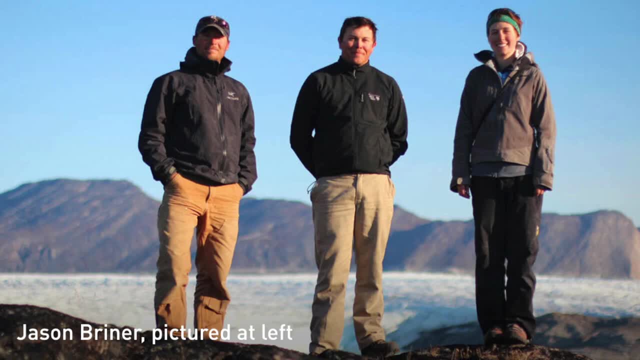 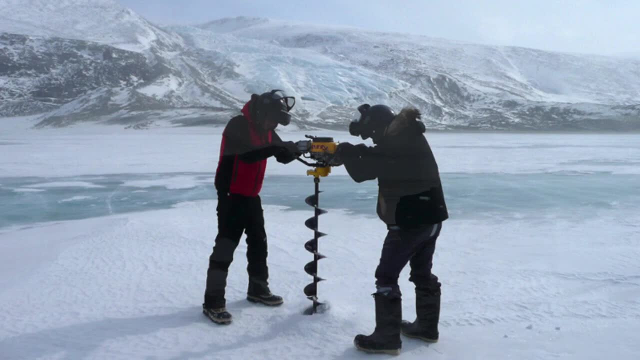 So we're publishing some new results in science, from Baffin Island in particular, that show that the ice sheet that existed over Baffin Island thousands of years ago, as well as smaller glaciers that exist in the mountains there, both responded to a very short-lived 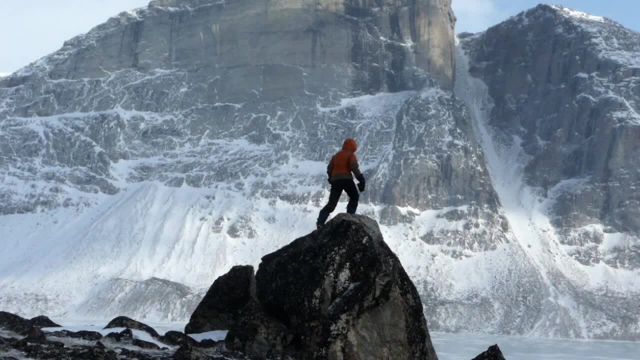 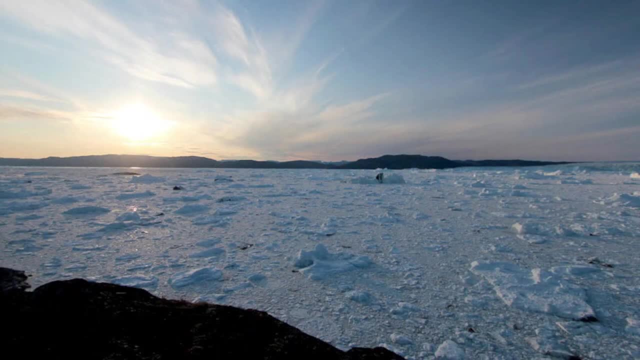 period where the climate was changing very fast. It's a very interesting finding because it's very similar to some findings we've had on Greenland. So we have a growing database of locations where the ice sheets and the glaciers respond quickly to this period of rapid climate change. 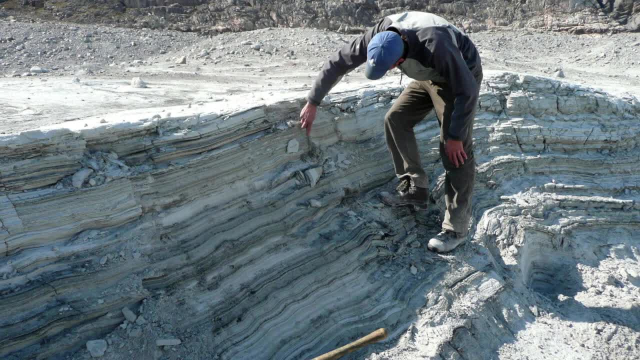 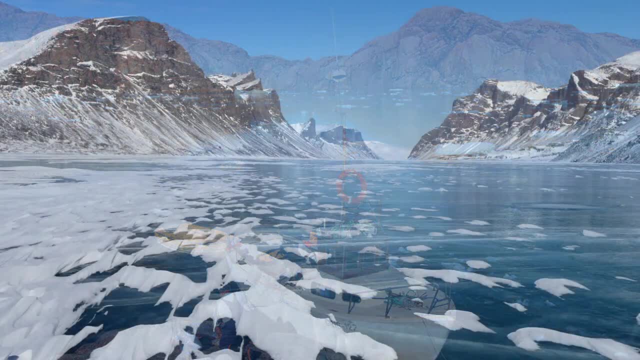 One of the ways that we hope our research will help with the current climate change problem is that our ability to forecast the future- the future of sea level rise, the future of how ice sheets change- largely hinges on models and the ability of models to accurately. 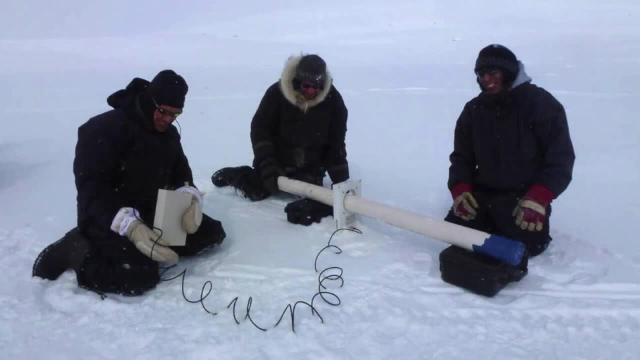 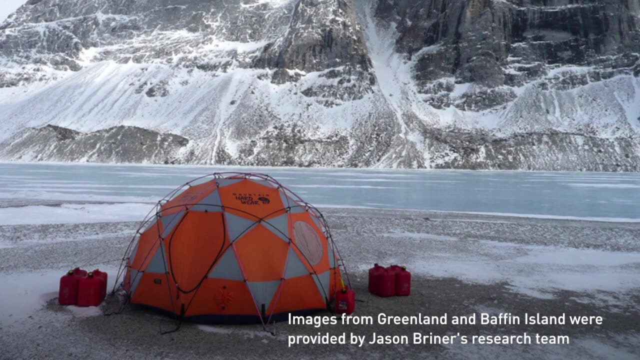 predict the future. The types of reconstructions that we're producing from our body of work ultimately help to improve these climate models. Thank you, Thank you.